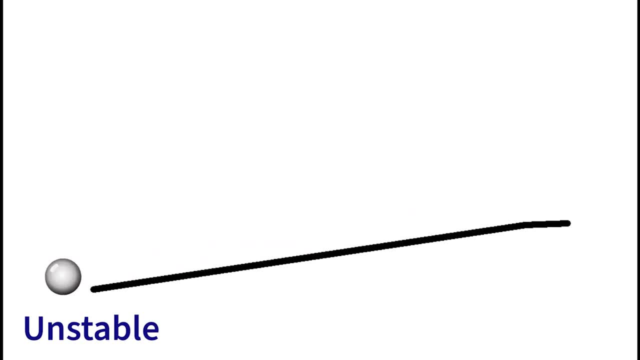 Here it doesn't even need a push and it will accelerate away faster and faster. If the marble sits on an odd shape like this, it's conditionally unstable, That is, it's stable or neutrally stable, unless it gets a big enough push and then it becomes unstable. 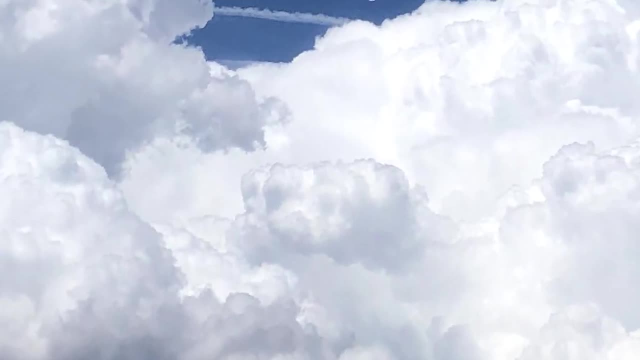 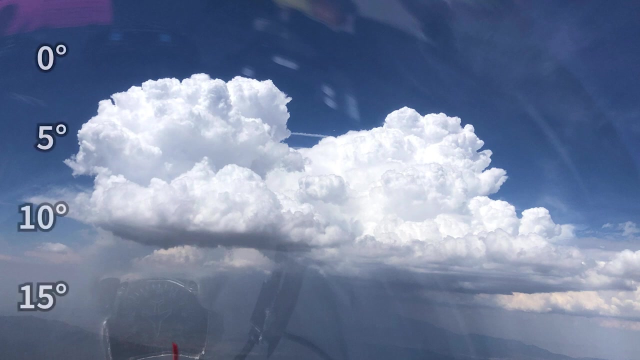 We can have similar situations in the atmosphere. In the same way that the stability of the marble is not so much dependent on the marble but the environment that it operates in, so too the atmospheric stability is a property of the environmental temperature gradient within a given altitude range. 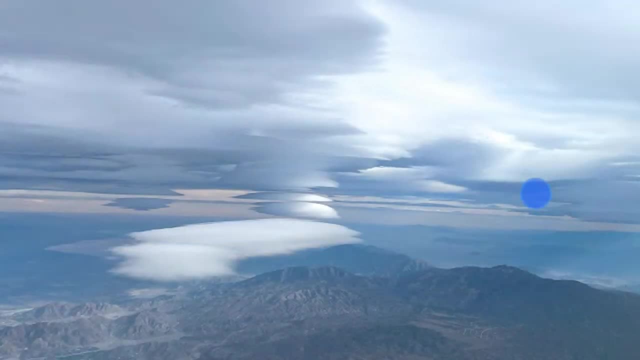 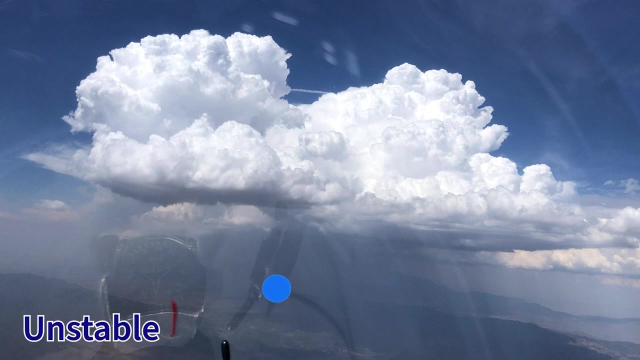 Our marble will be the parcel of air In a stable atmosphere. if a parcel of air gets pushed up or down, it will try to return to its starting place, its original altitude. This is what happens with mountain waves. In an unstable atmosphere, that parcel of air will accelerate away from a starting point. 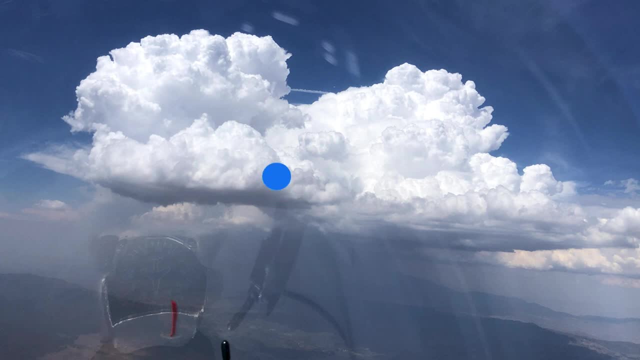 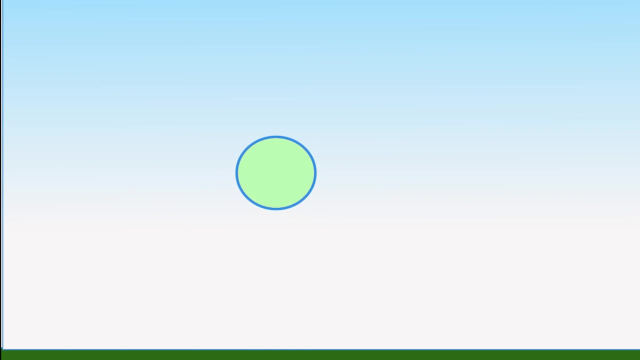 This is what happens when a towering cumulus develops and forms a thunderstorm. A key factor is the parcel's temperature change with altitude. When it's moved up, it will expand Its energy now distributed unnoticed, It will move down among a larger space, so its temperature will go down. 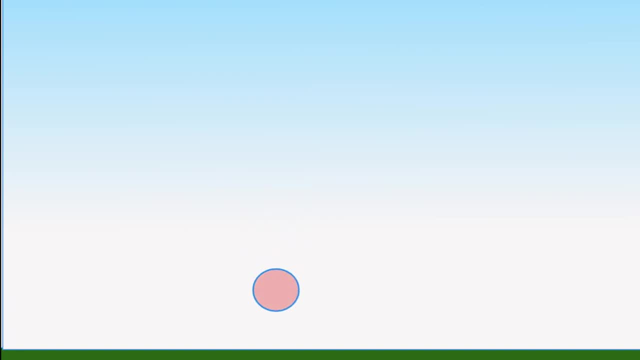 And the same in reverse. If it's moved down, it will compress and its energy will be in a smaller space, increasing its temperature. This effect of temperature change due to air expanding or compressing is called adiabatic. The rate at which the temperature changes with altitude is called the adiabatic lapse rate. 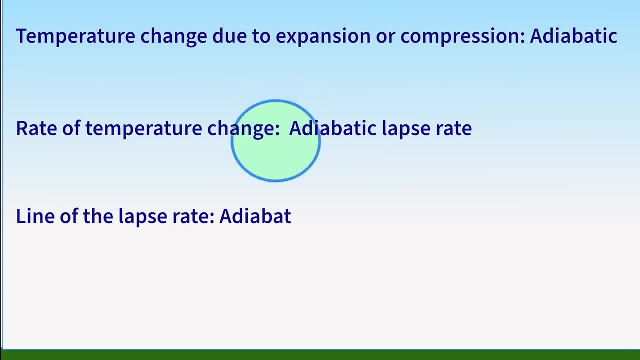 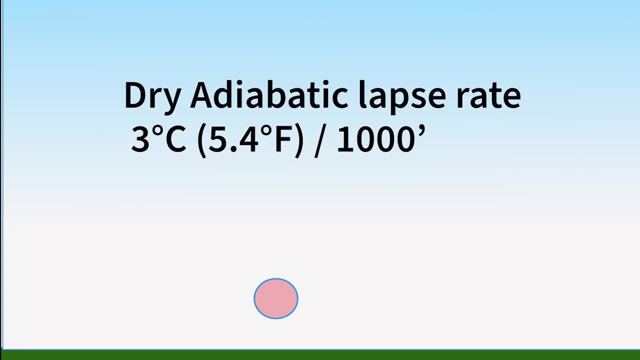 and when we plot it, the line is called an adiabat. This temperature change works for unsaturated air that is not in a cloud, in both directions at the same rate. that is, 3 degrees Celsius or 5.4 degrees Fahrenheit per 1,000 feet. 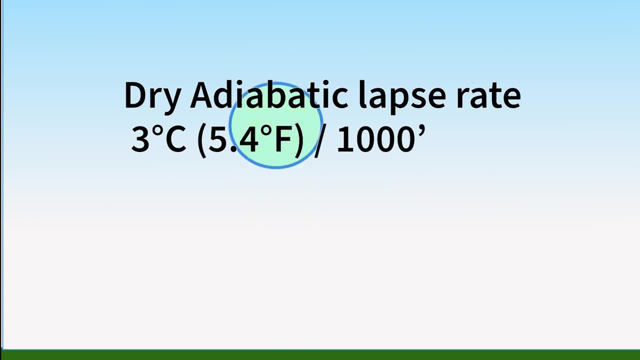 This is the dry adiabatic lapse rate. If we raise a parcel of air 1,000 feet, it will cool by about 3 degrees Celsius, and if we lower that same parcel of air by 1,000 feet, it will warm by the same 3 degrees. 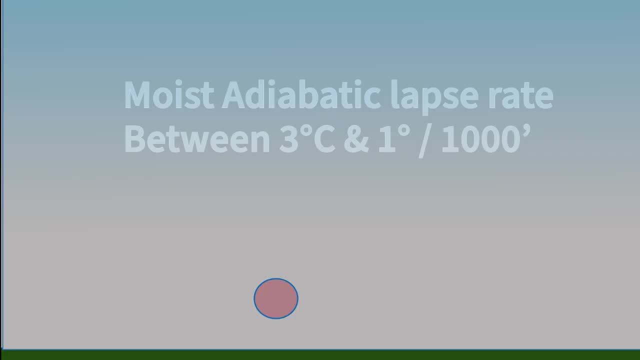 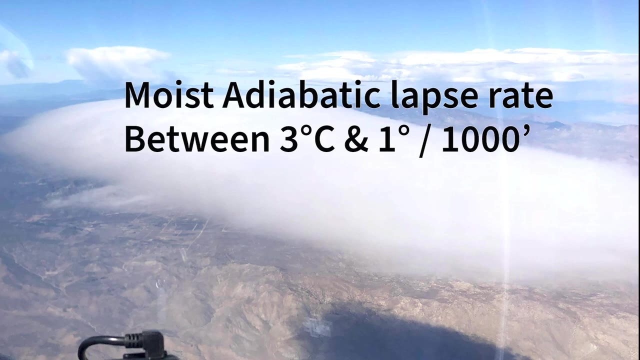 It can work for moist air too, as long as the droplets don't form precipitation in the meantime. The moist adiabatic lapse rate varies with temperature and ranges from about the same as the dry adiabatic rate of 3 degrees per 1,000 feet in very cold conditions. 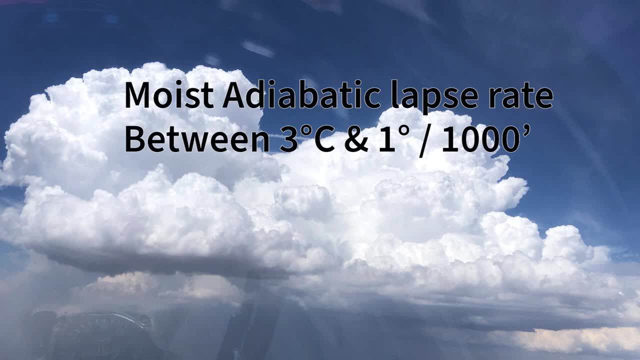 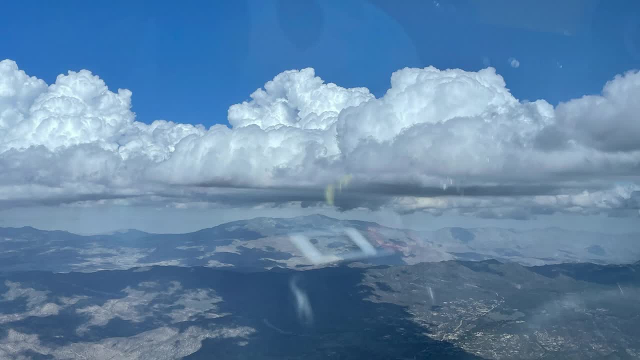 to about 1 degree Celsius per 1,000 feet in warm conditions. To determine where the atmosphere is going to be on this stability scale, we need to plot two different temperature trends on an adiabatic lapse rate chart, or SQT chart. 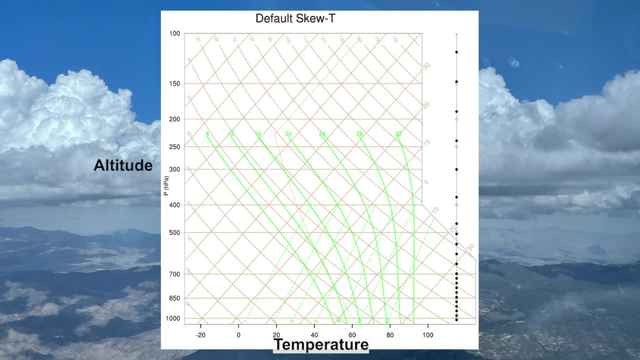 where altitude is on the vertical axis and temperature is on the horizontal, The environmental temperature at each altitude and the temperature of the parcel of air that's going to be displaced. The chart has lines that show the adiabatic lapse rate. We can plot the temperature of our parcel by drawing a line parallel to the adiabatic lapse rate lines. 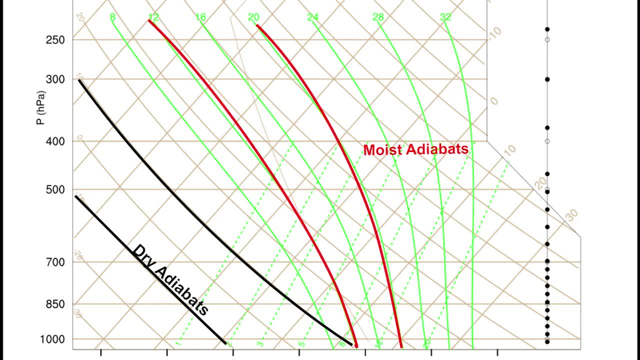 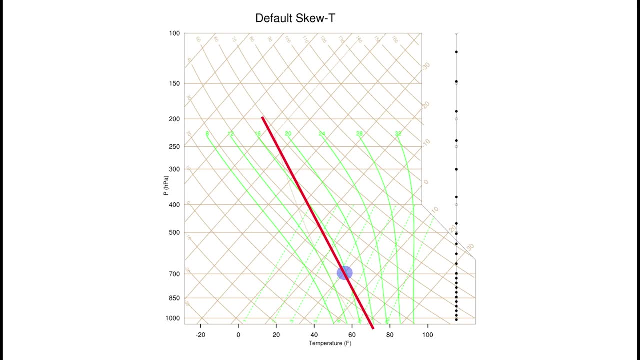 So what we need to do now is to displace the air in altitude and see how its new temperature compares to the temperature of the air around it at the new altitude. In the situation of a mountain wave, the air first flows down the downward or lee side of the mountain, where it compresses. 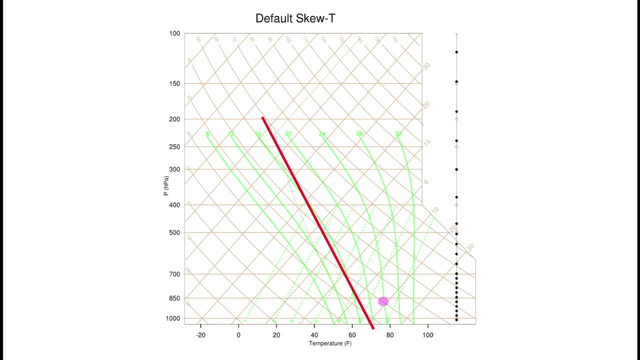 It follows the dry adiabat. we can see that it becomes warmer than the surrounding air so it will rise. It's got some mass and inertia so it's going to overshoot the point where it's the same temperature as the surrounding air. 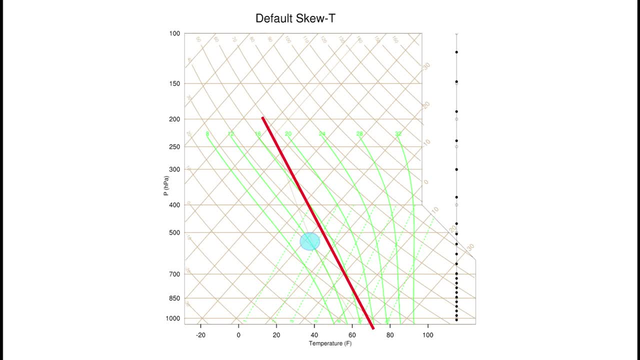 Now up here it's colder than the surrounding air and will turn around and sink, Overshoot a bit and repeat the cycle following the dry adiabat. This bouncing back and forth is what causes the waves to form If the rising air parcel maintains the same temperature differential as it changes with altitude. 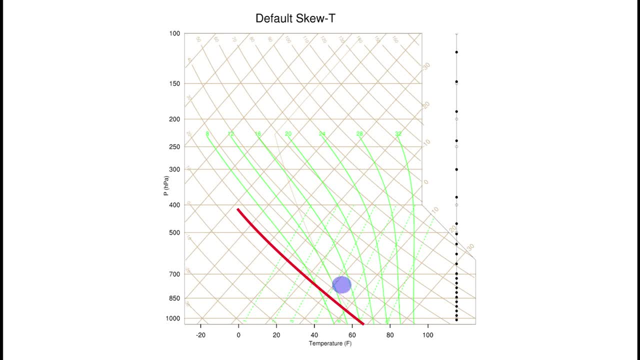 it will keep going at about the same vertical speed As long as that temperature difference exists. it is neutrally stable And if it's warmer than the surrounding air- more than it was when it started- it's going to keep rising and speeding up in the process. 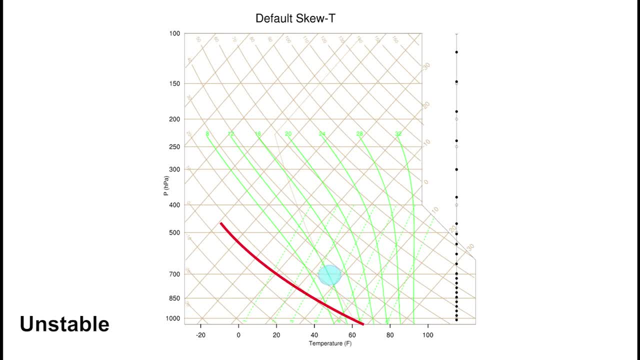 In this case it is unstable. Now the air can go from being approximately neutrally stable to unstable by having a cloud form. This is conditional instability. If the rising air cools to its dew point, a cloud will start to form Now, just as it takes heat to turn liquid water into vapor. you get that same heat back when the vapor condenses back into liquid droplets. That additional heat makes the parcel now moist, air cool slower, thus giving us the moist adiabatic lapse rate. Now eventually we run out of water vapor molecules to give up their heat.